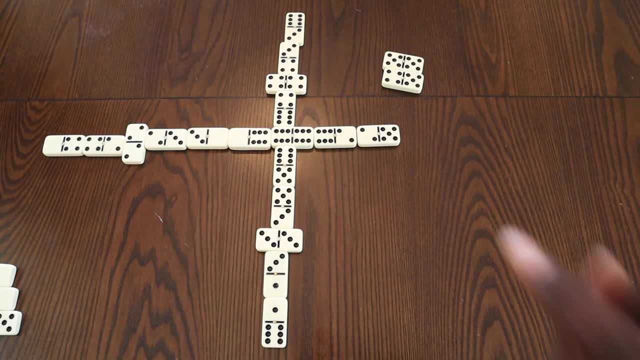 because all the sixes have been played. The opponent has two fives up there and I've just gone to the boneyard to draw this five. So the first thing that you want to do when you have a lot of dominoes in your hand. 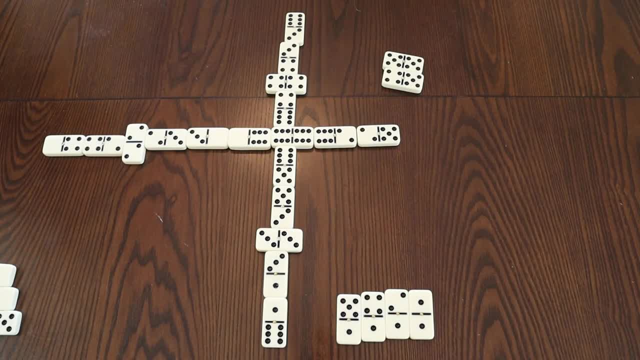 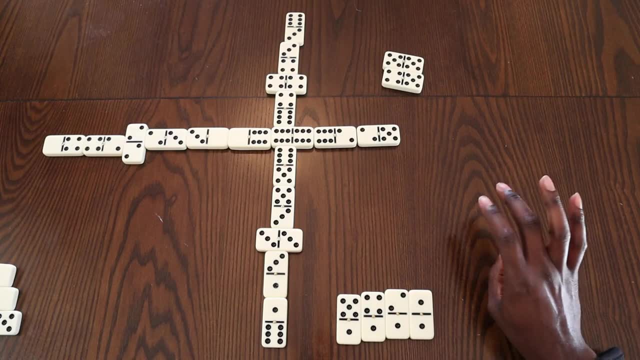 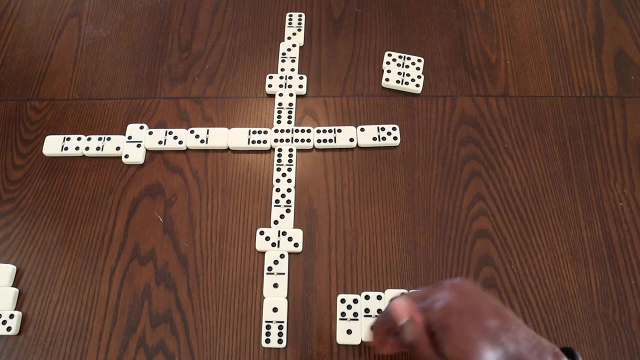 is: look at what you're strong with and then start counting dominoes. Remember, we talked about this in the last video. So you see, in my hand I'm very strong with the aces. So what I'm going to do is I'm going to count the aces right away. I see I have four. 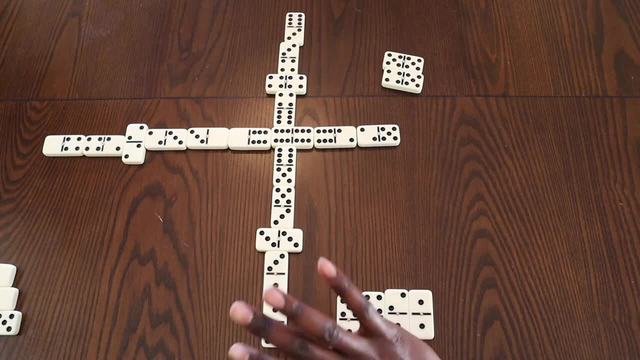 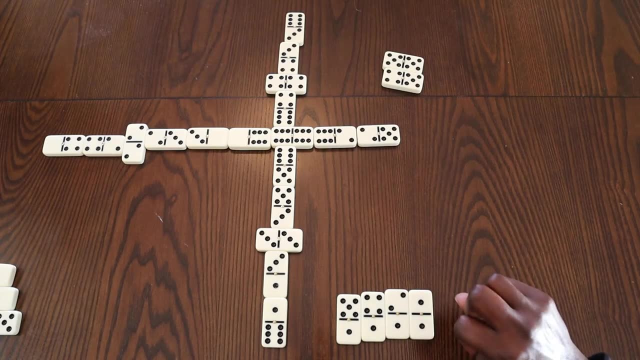 my hand and there are two played, So four, two, there's six. That means there's one ace left out there somewhere, Which one is that I have double ace. I have ace two, ace three is played, Ace four: 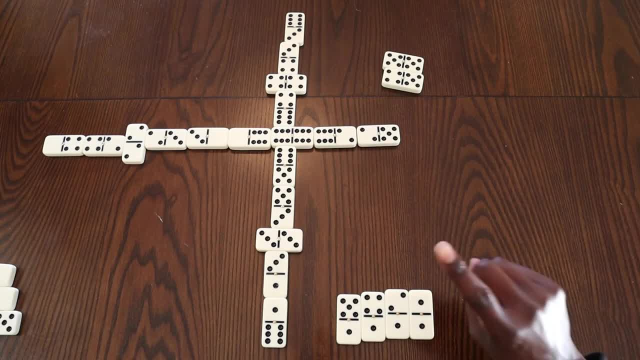 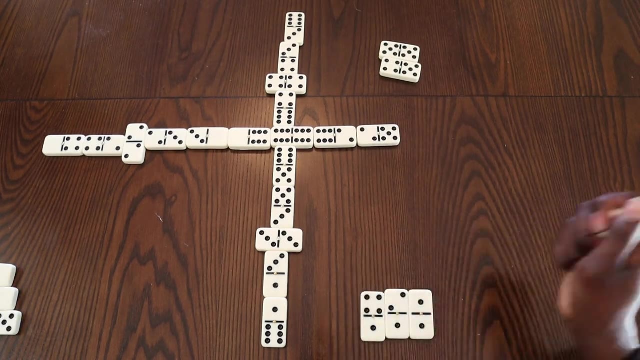 is here, Ace five is here, Ace six is here. That means we're missing ace blank. So ace blank is the domino that is out there somewhere. So even though I have, I've just drew this one play with the five I'm going. that's my only play I'm going to go with. 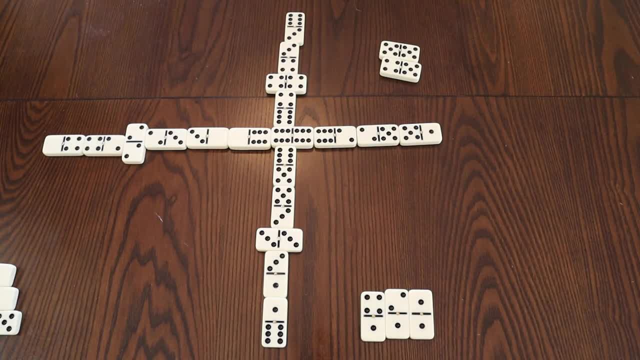 that, and I'm going to play that convincingly, knowing that there's only one ace left out there in the board. Now my opponent: they have double five and five, four in this instance. So now they can't play. So what do they do? They go over here to the boneyard and they pull one, They pull. 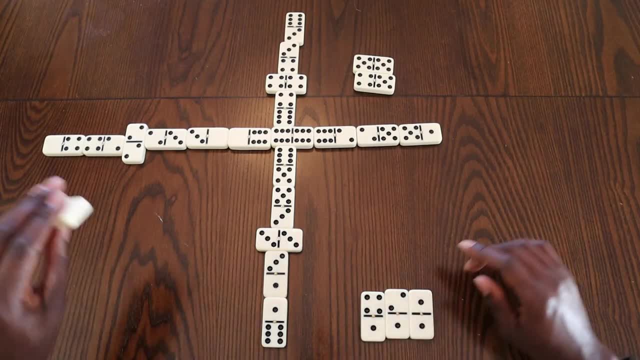 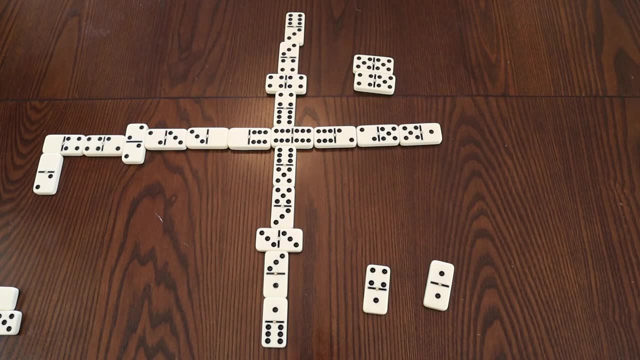 blank two. So they're going to play the blank two. And then right back to my hand, what am I going to do? I'm going to hit that two, and hit it quick Right, Because again I'm going hard with the dominoes that I have. I'm strong with aces, So 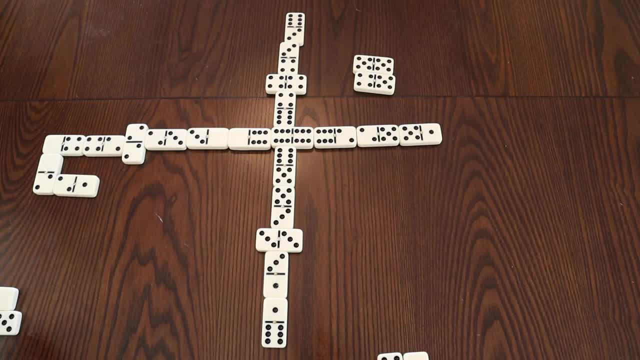 I'm forcing those aces. Now the opponent. what are they going to do? They're going to go right back to the boneyard, They're going to draw a double blank And then they're finally going to draw blank five. 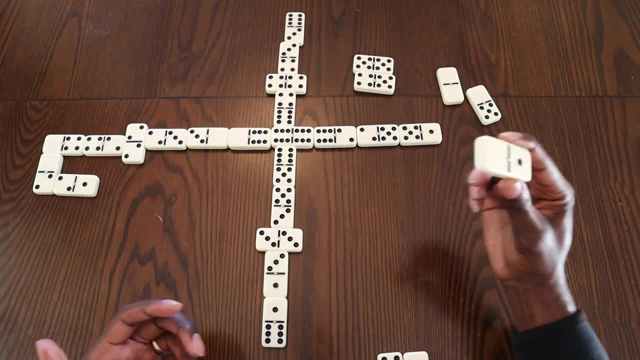 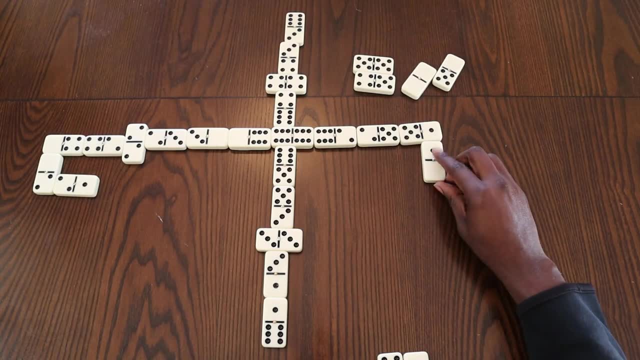 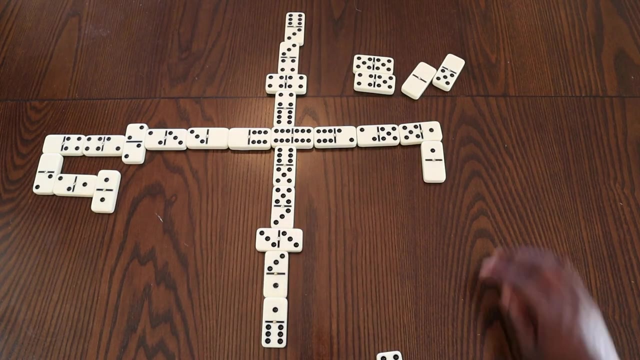 So now they're in the boneyard And then, lastly, they draw the bone. we were looking for the ace blank, So they're going to play that ace blank. So now, what do I do? I come immediately and play double ace. And then what are they going to do? They're going to maybe play the five right there. 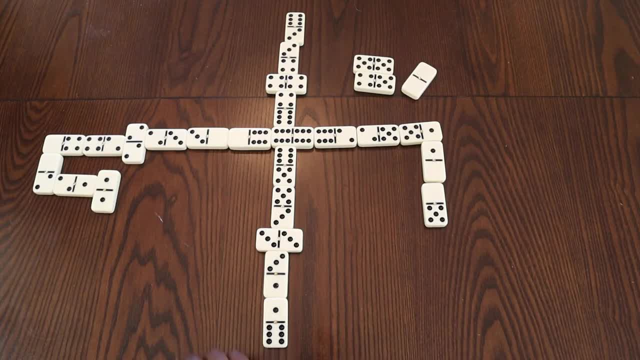 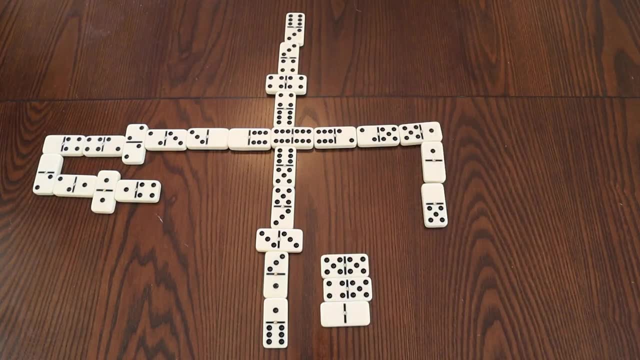 trying to cut off something or just drop a heavier domino, And then I'm going to go out with the ace four. And what I'm going to do? I'm going to collect these dominoes from their hand. I'm going to take. 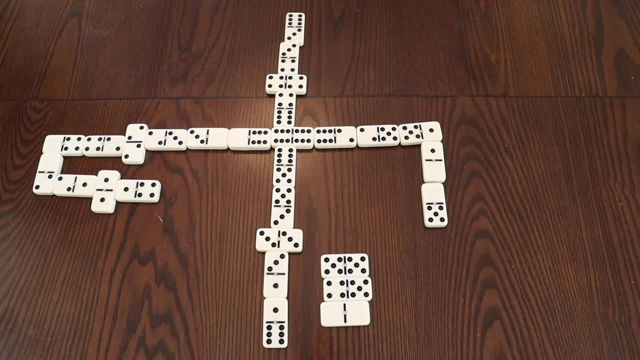 20 points. So you saw how that went. I went from having four dominoes in my hand and they only had two. Yet I was able to turn the tables on them because they sent me to the boneyard and loaded my hand up. So what did I do? I counted the board to see what I was strong with. 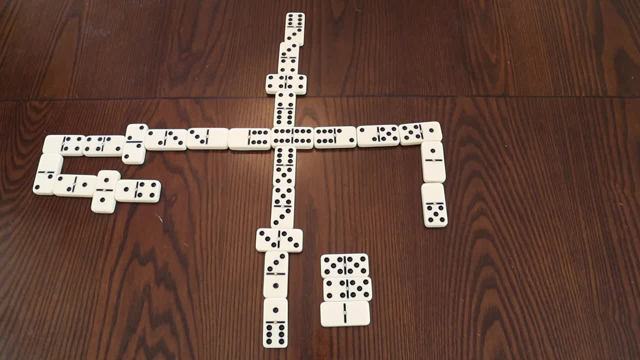 looked out for the one domino that could stop my momentum, which was the ace blank, And then I played my hand accordingly, sending them to the boneyard. Now, since they equipped me and turned the tides, took their domino from them and exited the hand with 20 points. 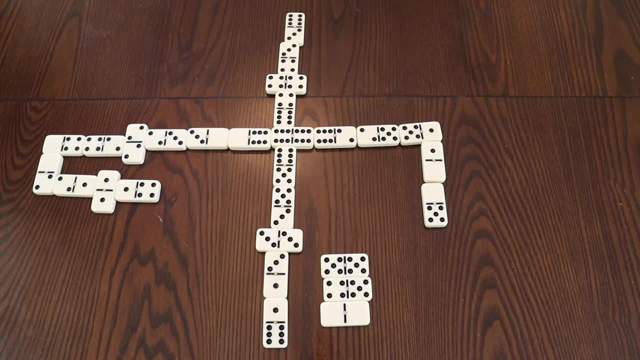 Hopefully you were able to follow along what happened in that video and that scenario And now you know what to do. when someone sends you to the boneyard, fills your hand up, The first thing you do let's go over it one more time. You count the board to see what you have. 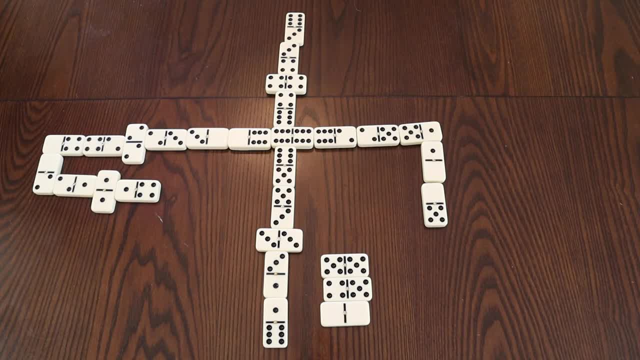 most likely don't have, and you start playing that to turn the tables on them, sending them to the boneyard. So again, this is what you do when you go to the boneyard, your hand gets very full, you play it to your advantage and you want to then put the pressure. 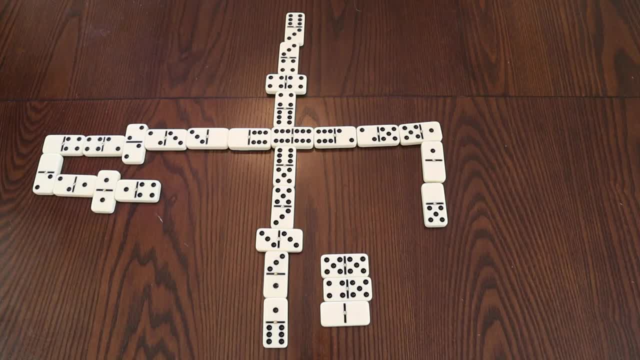 on the opponent. Hopefully you enjoyed this video and remember to like and subscribe, as this helps the channel continue to grow. Thanks for watching and I'll see you guys in the next one. Subtitles by the Amaraorg community.